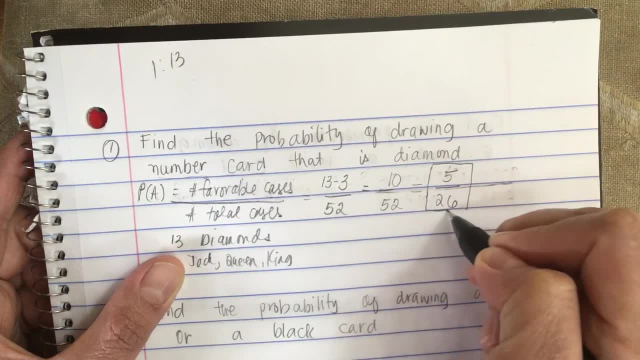 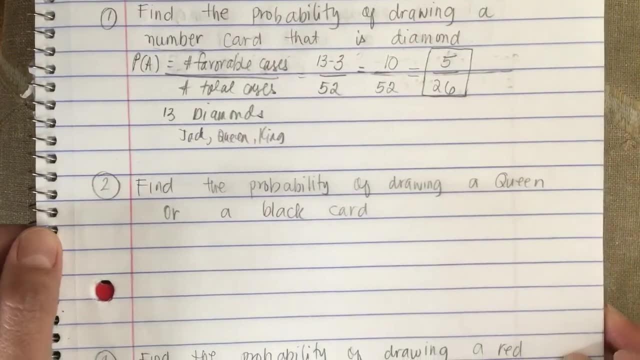 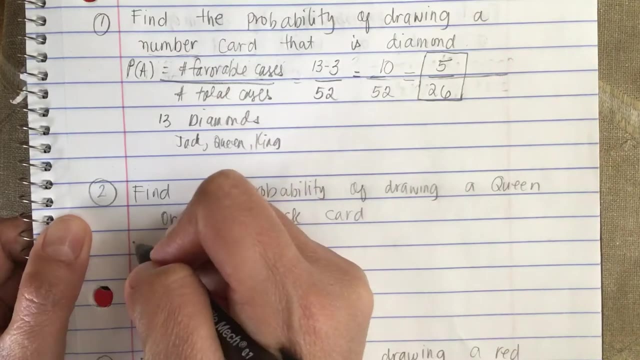 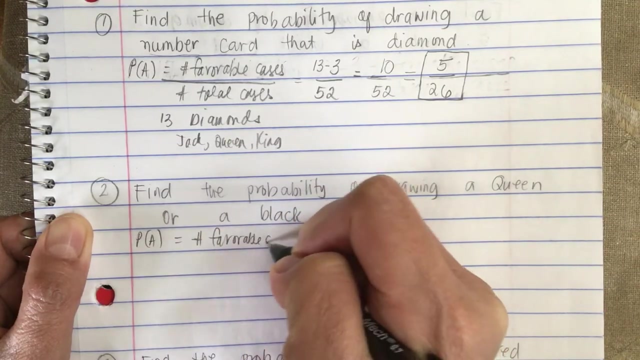 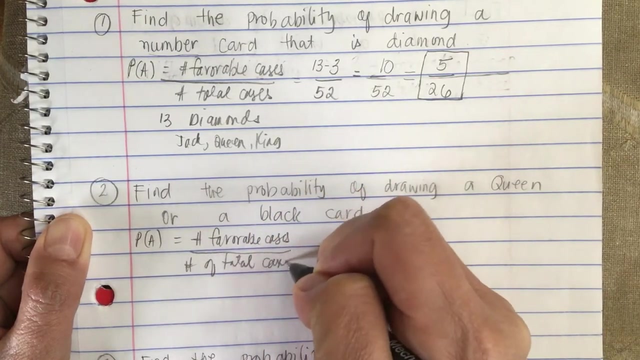 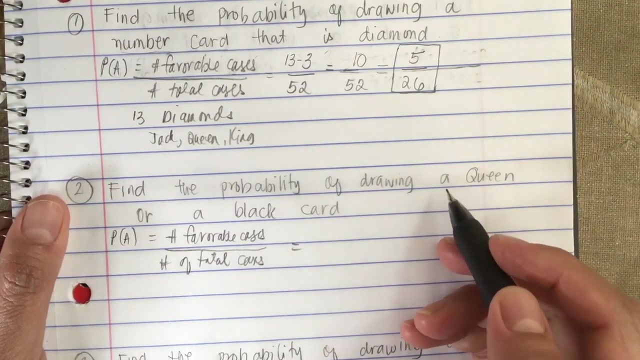 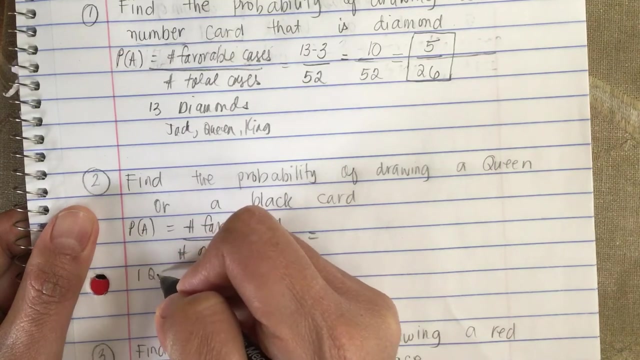 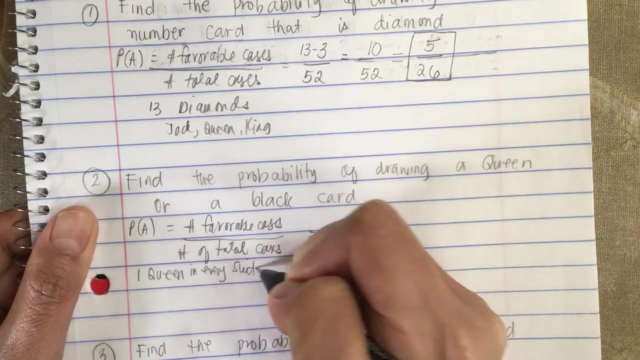 find the probability of drawing a queen or a black card. so again, the probability of any a is equal to the number of favorable cases all over the number of total cases. so let's examine this. so, drawing a queen, now there is one Queen in every suit, one Queen and every suit. so total Queen is four, because one for spade, one. 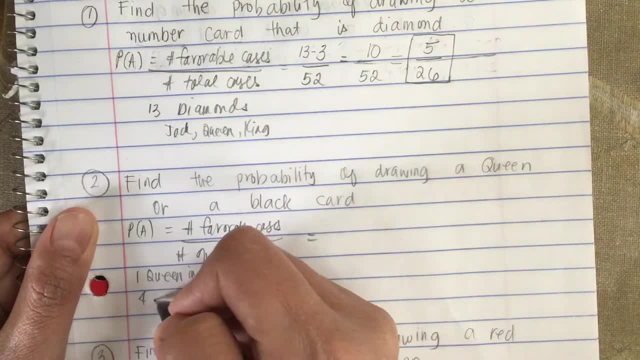 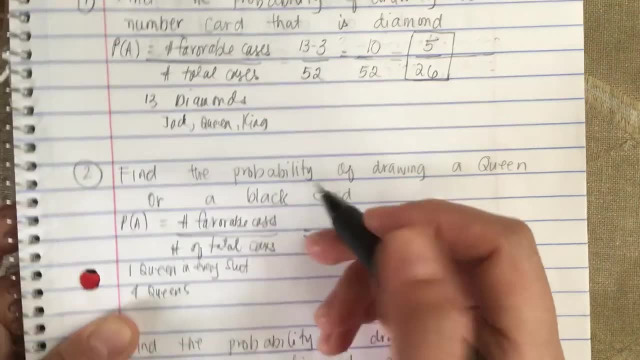 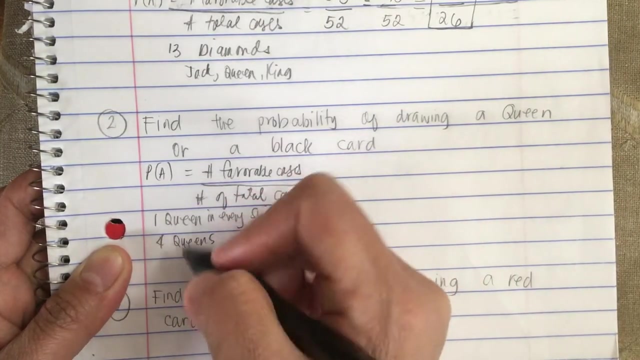 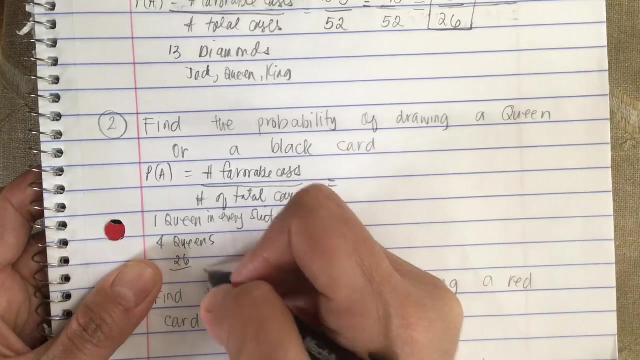 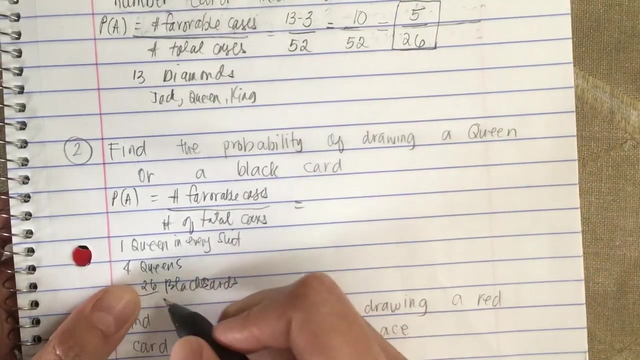 for club, one for heart and one for diamond, so four queens in total. so now a black card. so there are 52 and half of it is black: club and club and spade. so that means that there are 26 black cards, black cards. so now there are 26 black cards and now we have to add the queen. 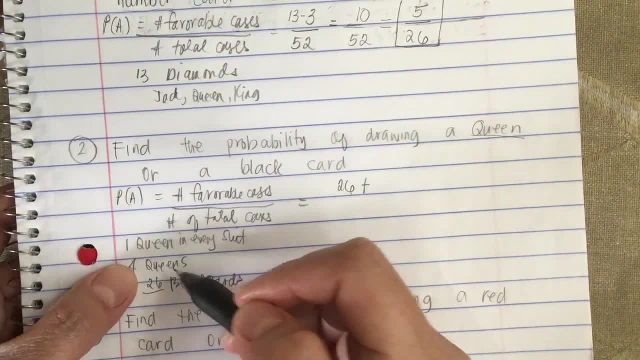 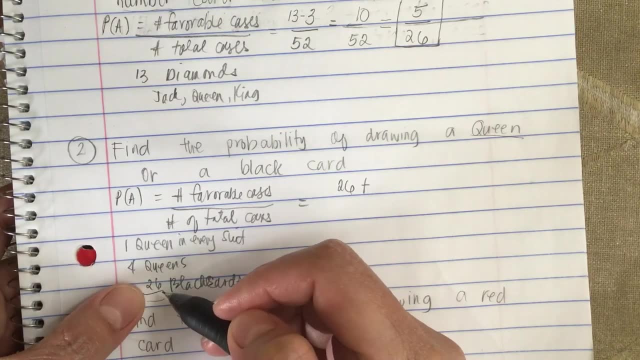 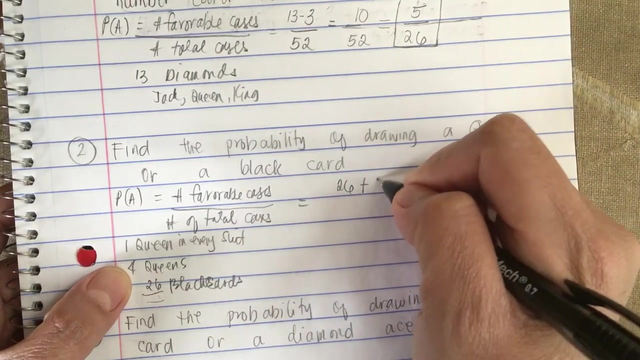 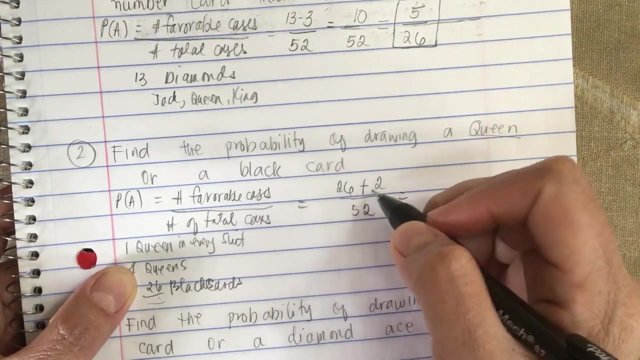 so now there are four queens, but two of the queens are already counted in the black cards: the queen of club and queen of spade, because those are blacks. so that means that we have to add two more: the queen of diamond and queen of hearts. so over 52, or 26 plus 2 is 28 over 52. 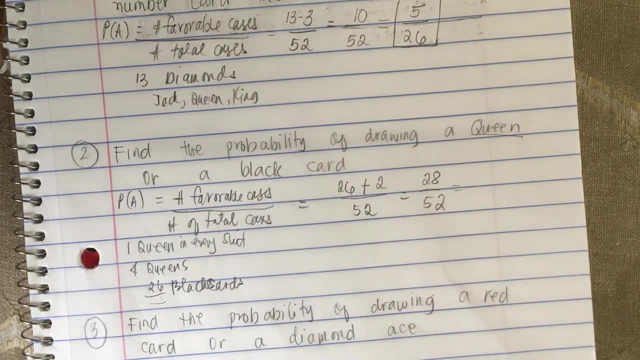 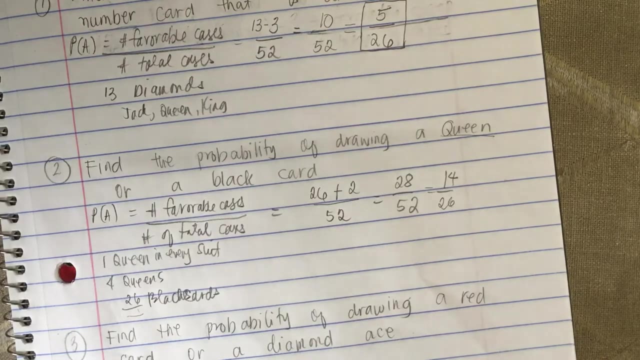 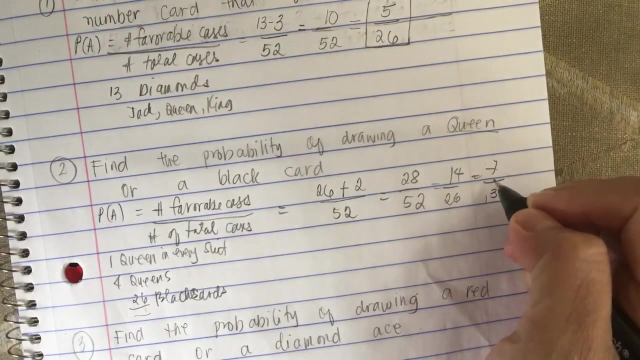 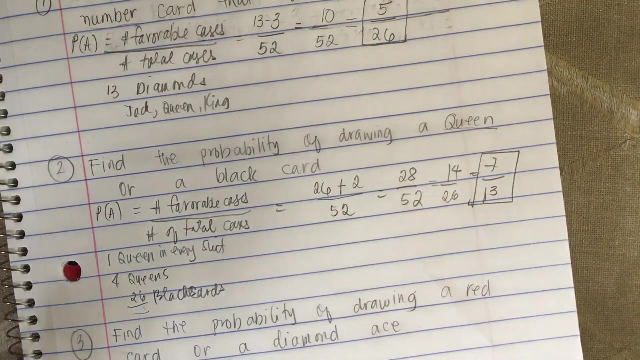 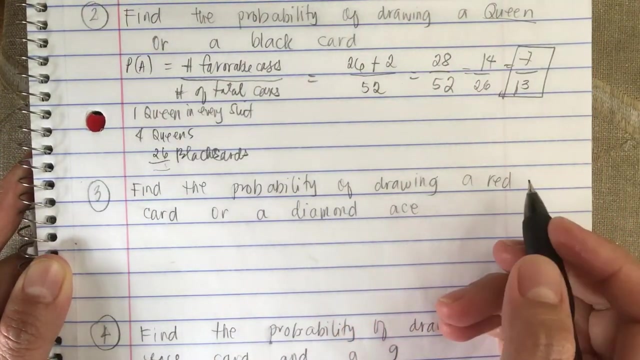 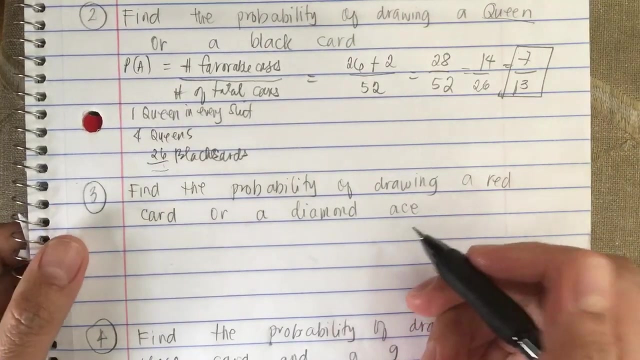 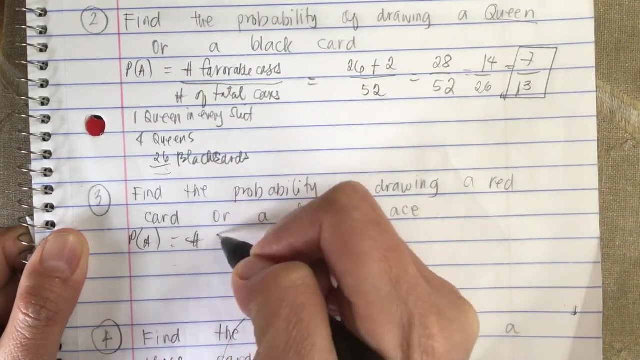 or let's reduce this to. so if we reduce it by two, it's 14 over um 52, um 26, so and it's still even so, this is 7 over 13. so next one find the probability of drawing a red card or a diamond ace. so there are one half or 26, so probability of a is equal to the number of. 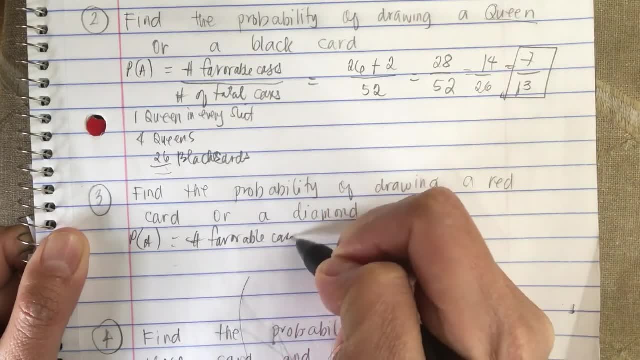 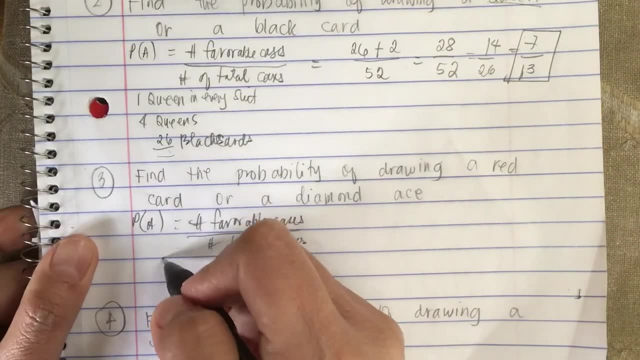 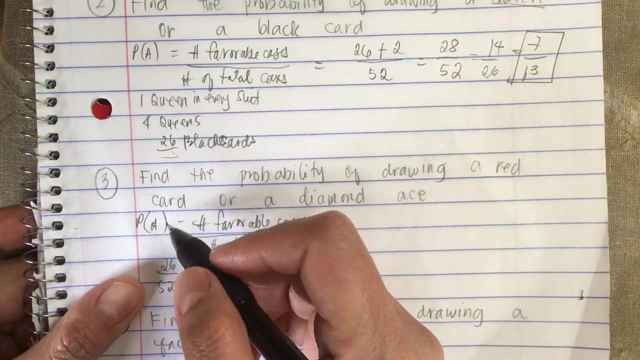 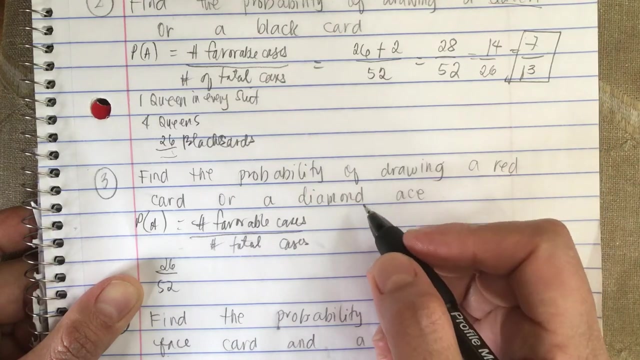 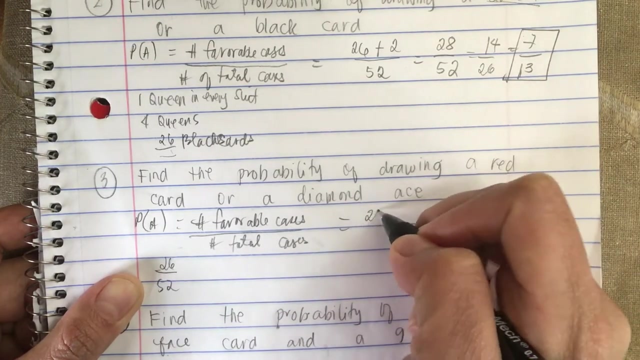 favorable. favorable cases all over the number of total cases. so there are 26 over 52. um red card. so red cards are the diamonds and the hearts. now we add the um or a diamond ace, and it's already a red card. the diamond ace is already a red card. so this is 26 over 52, or this. 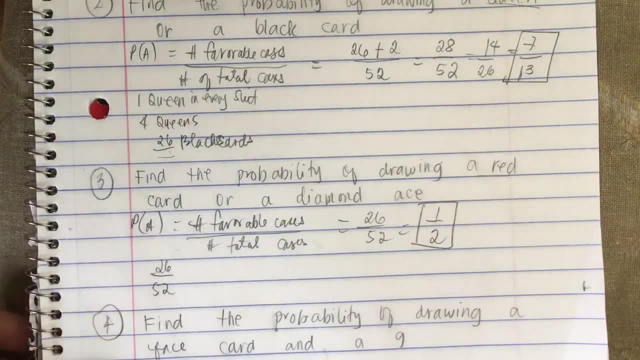 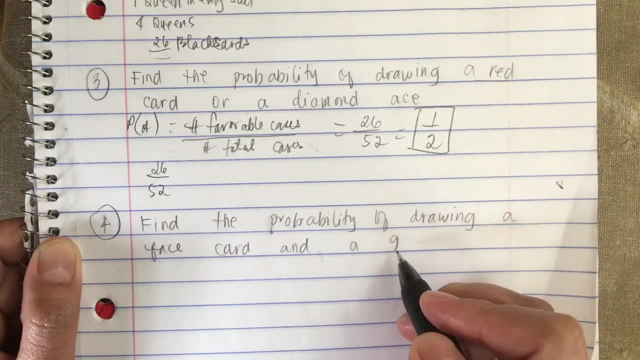 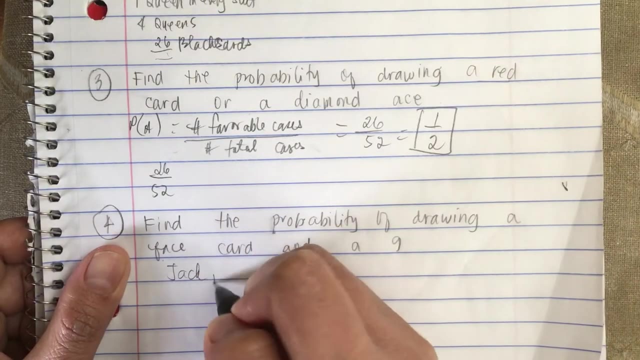 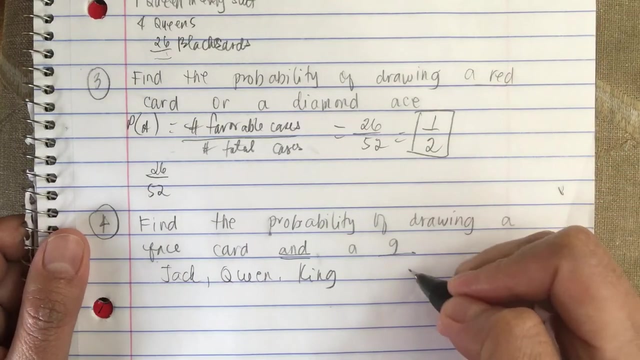 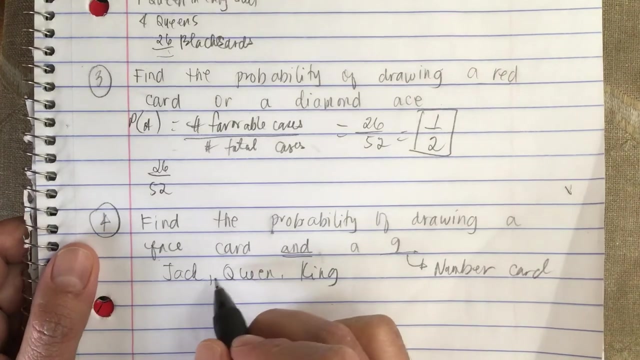 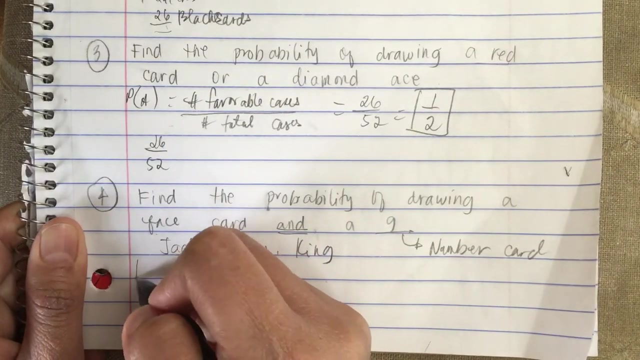 is one half. find the probability of drawing a face card and a nine. find the probability of drawing a face card and a nine. so a face cards are jack, queen and king. so a nine is a number card. so this is a number card, number card. that means a face card and a nine is not a possibility. so this is the probability. 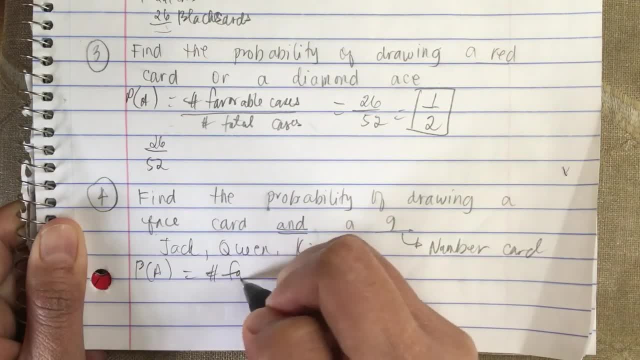 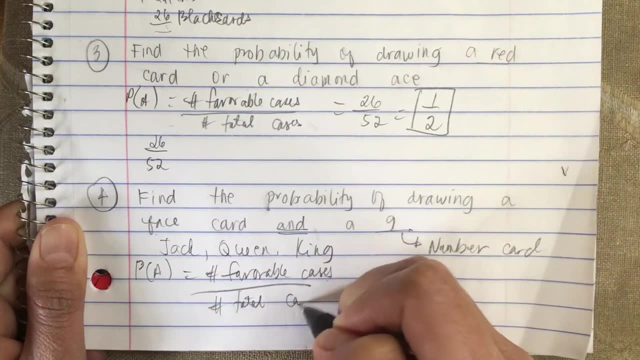 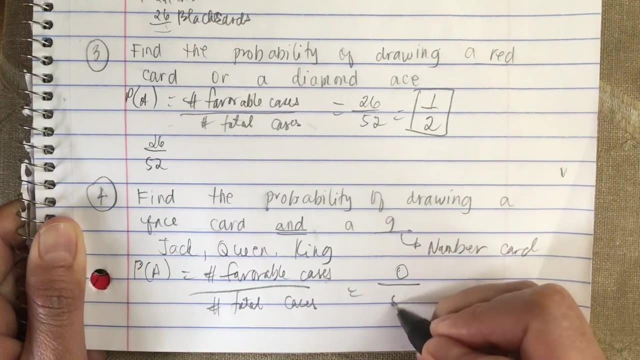 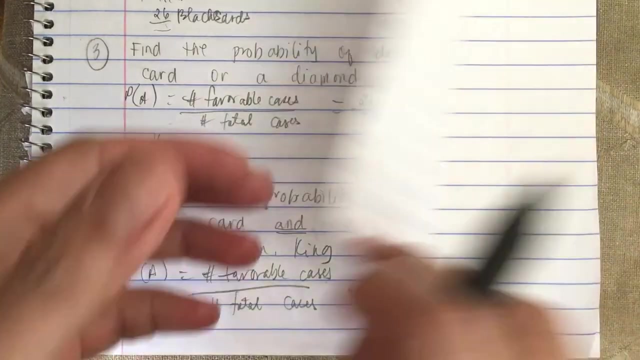 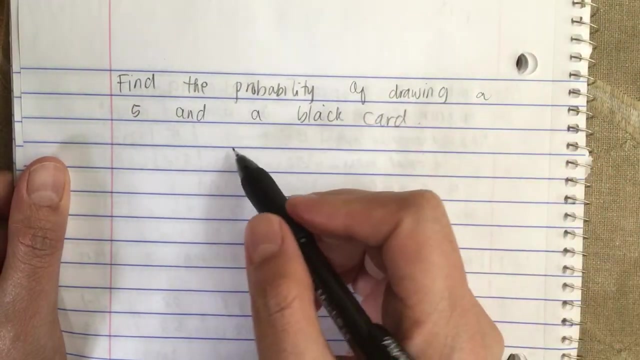 of a is equal to the number of favorable cases all over the number of total cases and a face card and a nine is there's no probability. so this is zero out of 52. so this is zero. find the probability of drawing a five and a black card. so